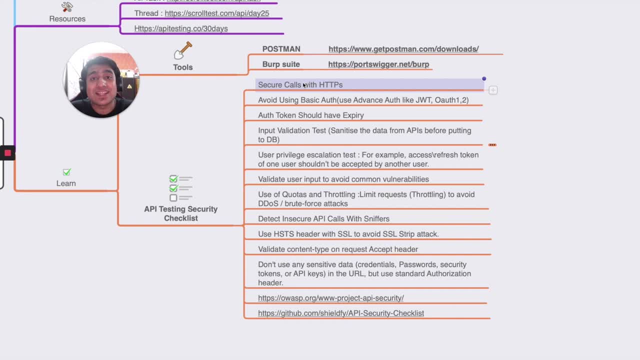 doing api testing. uh, those requests should be secure and they should be behind the sdpps, right? if you are going to production, make sure though the in even the internal calls, if possible. guys, this is important i'm telling you with my experience. i have your experience. if you have internal codes in your micro services, make sure they are sdpps, because a lot of time 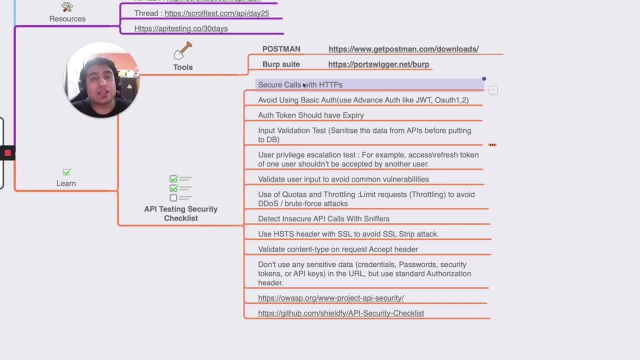 people. uh, compromise certain systems and insecure requests hacked very easy, right? so make sure you do that. avoid using the basic auth guys. this is one of the basic mistake that i have done, like in the micro services. when we were testing of microservices, apis right and they have basic 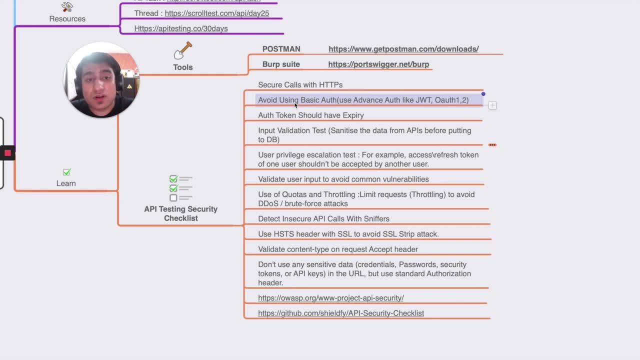 auth and that basic auth was compromised lots of times. so i would recommend you, if you can possible, go with blr token java, awt auth one or two, something like more advanced and more uh. or you can go with digest, also right, more advanced. avoid basic auth, just that. that's the simple, simplest point, right um about means. 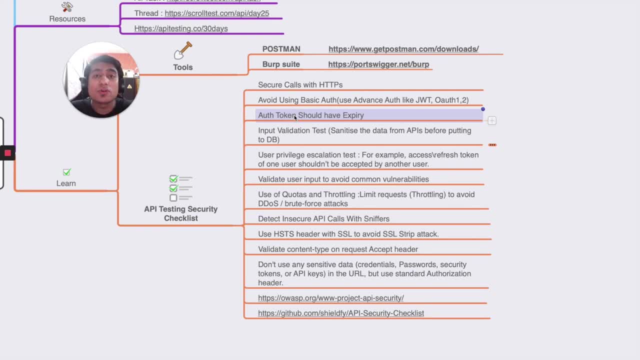 all the authentication token or any kind of authentication that you're using, right, they should have certain kind of a expiry with it, right? i've seen that login apis. their expiry is again six months, seven months. this this makes it doesn't make sense, right? uh, i would recommend you. 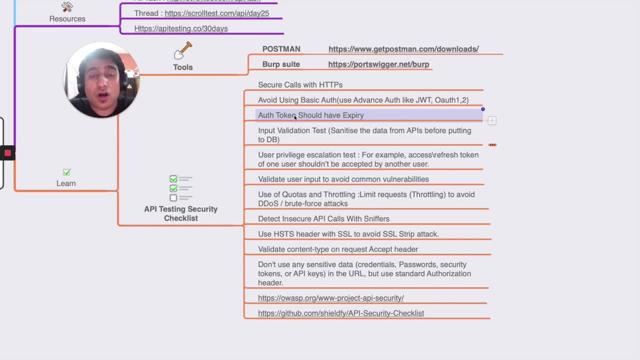 check it out, as it's, uh, api tester which we, uh, we should be checking these things right. uh, we should know that authentication should have expiry if we want to check it in a security way. security testing, right, right, input validation again, this is one interesting one. suppose you have a username. 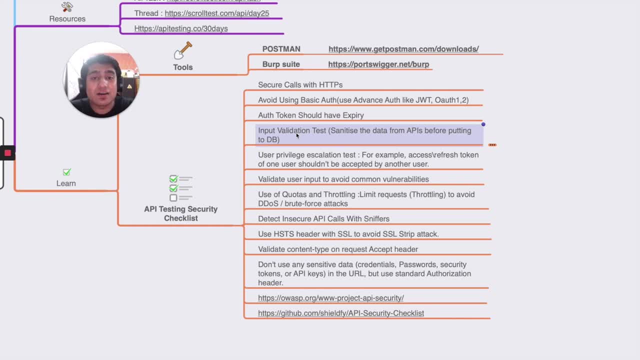 password, api that you are testing. you should have api or you should have input validation. basically, standardization means i cannot add anything malicious, like exorcist attack or anything like this, and sanitize your data in the backend. make sure you check this and tell your backend developers to sanitize everything. 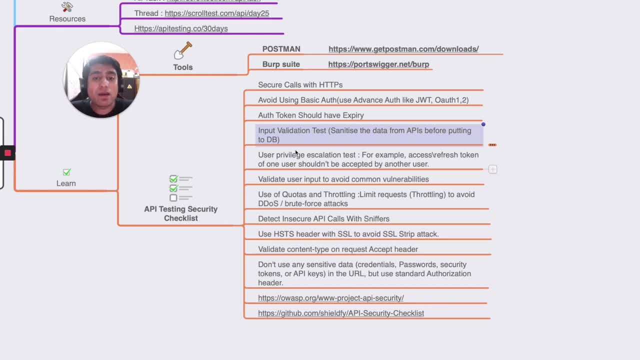 that you are. that is coming from any kind of a input right. uh, user privilege escalation test that you can test, basically access or refresh token for one user shouldn't be accepted for one another users. i'm going to tell you about the interesting story here, guys. uh, i have hacked. 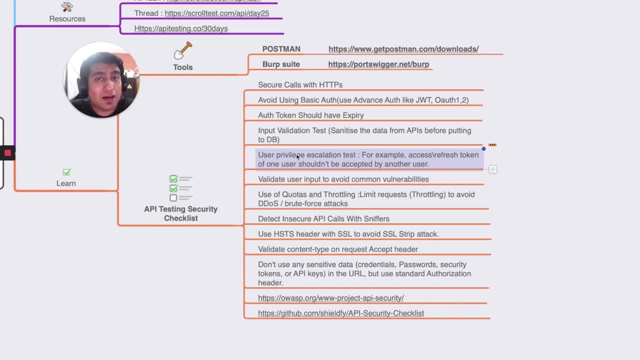 one of the la, one of the largest uh webinar platform, or funnels platform, if you know, and they have given me a very great bounty due to this uh, they have the privilege escalation, or i don't. generally we call it right indirect object uh references. so while i was testing their 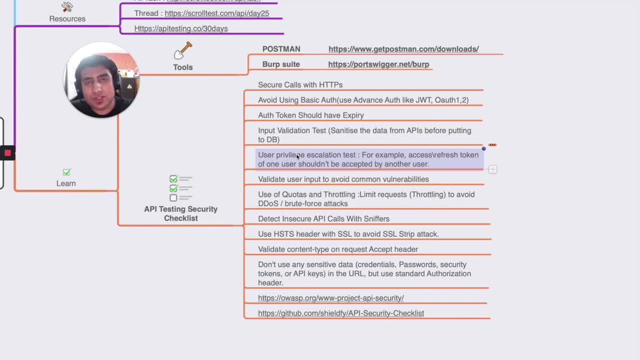 apis i was able to access few of the users. even i was able to change the plan to pro basically lifetime access of their plan, which cost around thousand dollars. and also they have provided very decent, very decent, uh uh, very decent, you can say- bounty for this one. so api testing security is 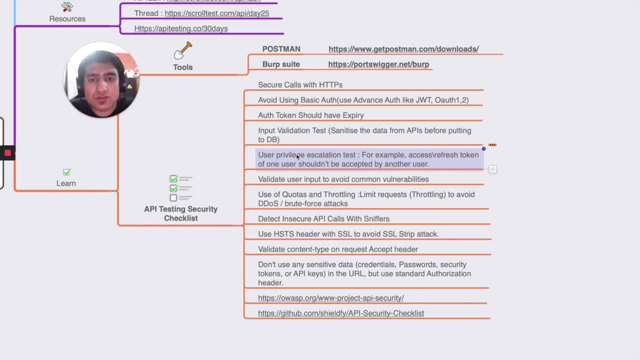 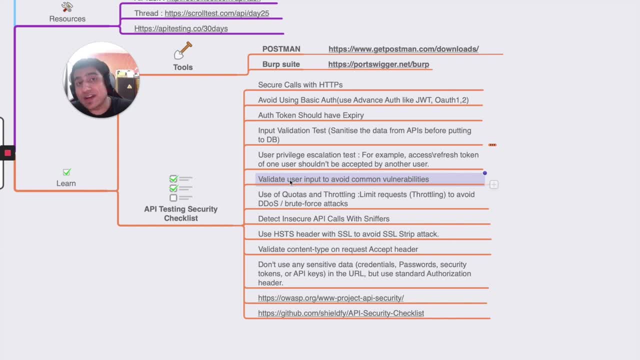 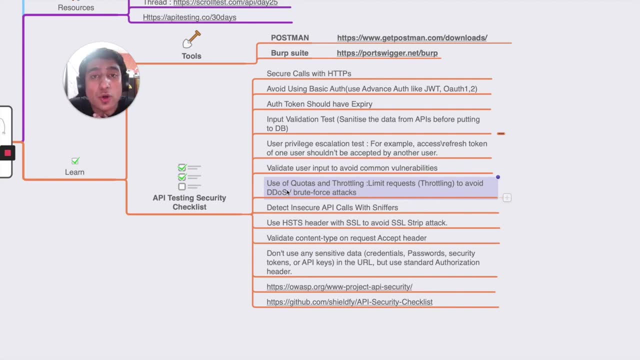 avoid common vulnerabilities. that is important. you can go to os top 10 and check for the vulnerabilities. uh, this is important one. again, the point here is about the quotas and timing throttling the request. so make sure, uh, if anyone wants to do brute force thing or something like this, your apis gives four to nine too many request error or something like. 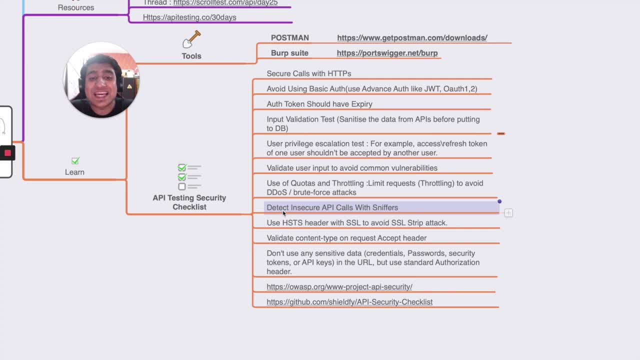 this, this is properly handled. detect the insecure api calls with snipers. uh, basically, any kind of a known secure call is coming to your back end at all. uh, you need to make sure that, as a api tester, these things are handled properly. uh, this is one other word. uh, another important is as as hsts header. 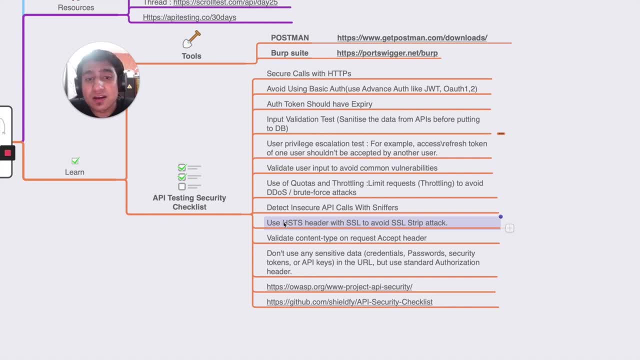 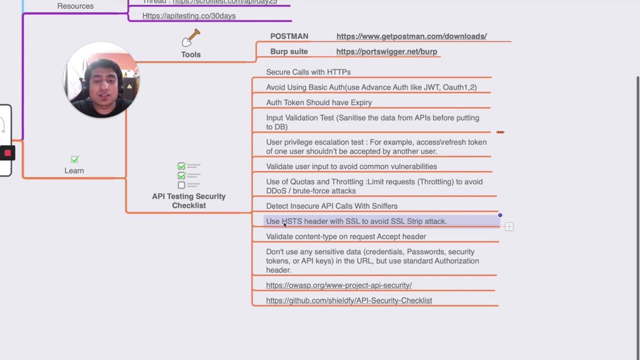 to basically avoid the ssl strip attack. this is one of the attack uh that uh in the sdps. basically. so, uh, if you can use it, you can uh tell your developer or any kind of back-end developer printer, but we use these kind of ssds header so that, uh, you can avoid this test, uh avoid. 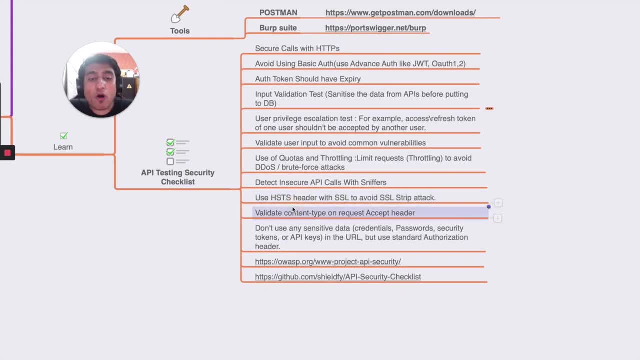 this kind of misbehavior right. you can validate the content type: adults and all right. don't use any sensitive data like credential password security extra uh in yours uh, and use only the standard authorization headers, right uh. sometimes people uh whenever they are creating apis, right, so they add their custom made headers or sometimes they pass the headers information. 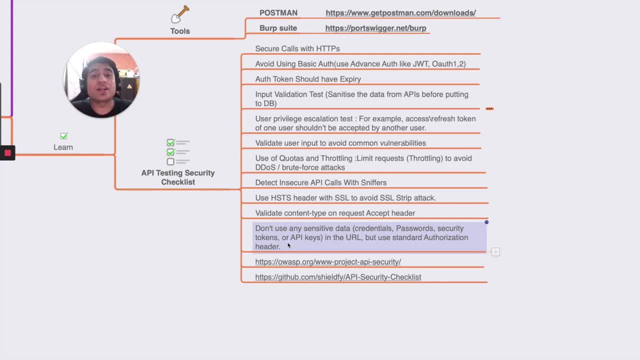 something like this. avoid it, completely avoid it and as a api tester, you should be ready that don't do this kind of stuff. uh, use standard authorization methods. that is important, right? uh, i will highly recommend you to watch those. uh, basically, i'm going to open these two links. these are very 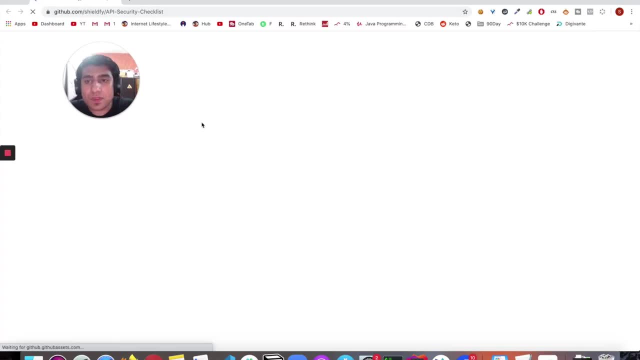 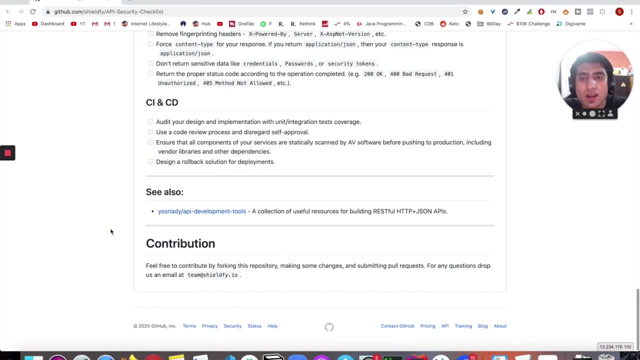 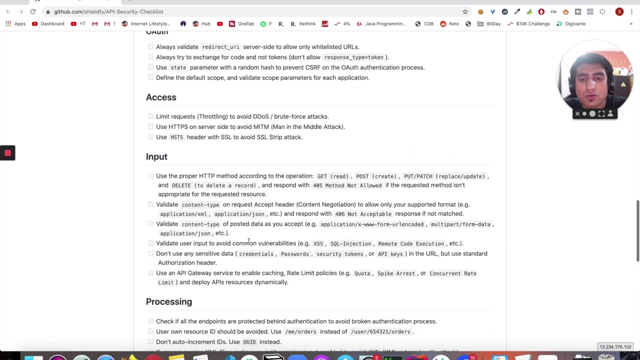 much important, so let me open this one for you, and this is api security checklist and, uh, you can go through the whole list. it is very interesting one. uh, a couple of few things they have mentioned about this: how to avoid browse for tag. don't use basic code right in how to validate. 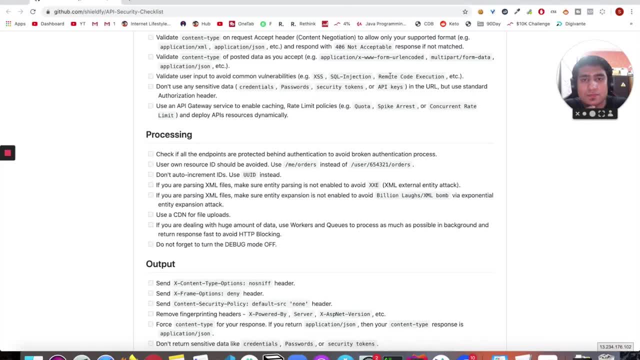 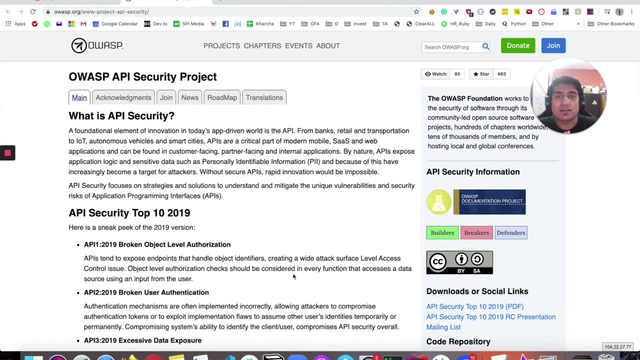 input for sql injection, remote execution, right, so that you can do, right. so, uh, let me open this os link, so os limp, uh. basically. uh, in this paragraph they have given you about this some of the major important points about the api security, right? uh, if you are already a security engineer, you already know about that. os provides lots of. 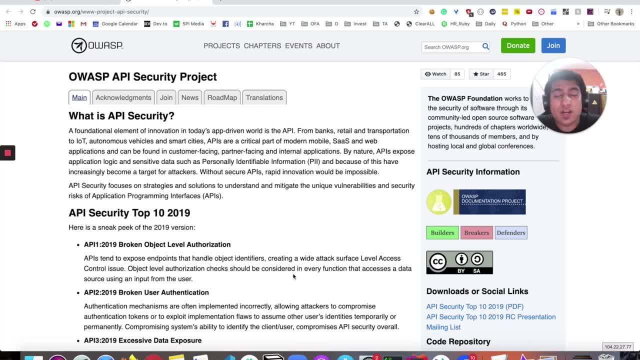 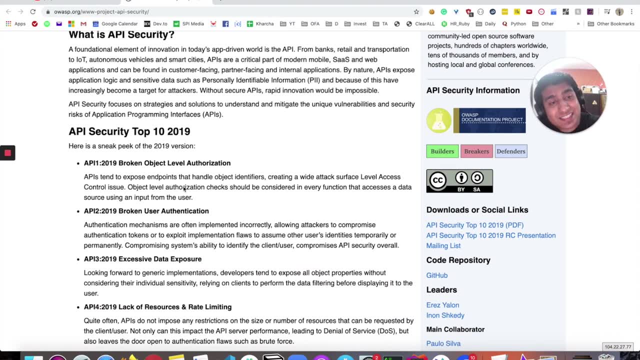 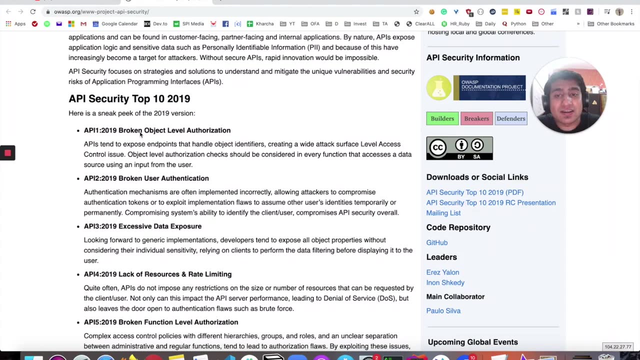 resources of and as well as tools about the secure security right and this is uh the top most. you can say api security dot top uh type of attacks they have discussed here in the. so in 2019 we have like uh most uh like broken object level authorization right, these kind of attacks, broken user. 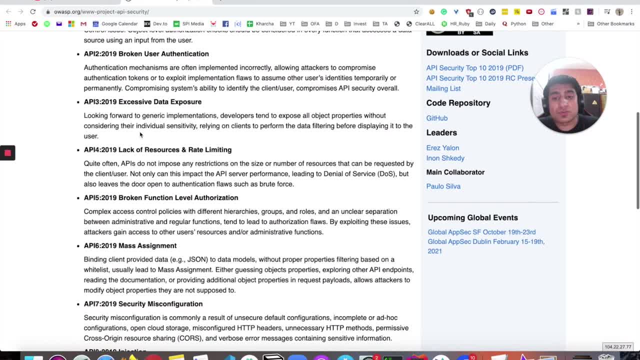 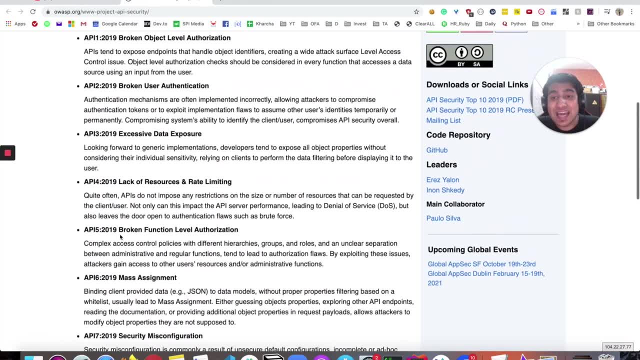 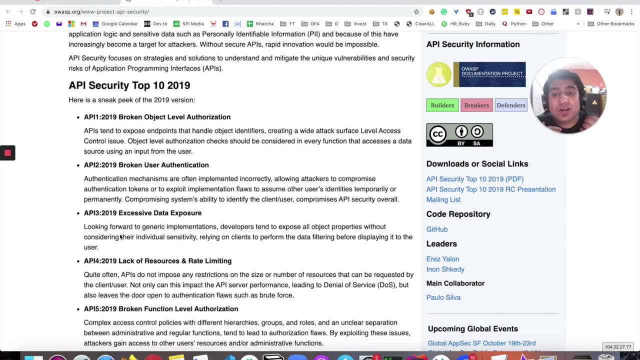 authentication, excessive data exposure, lack of resources, broken function, mass management, security, misconfiguration, injection, improper access- these things right. so these are 10 of the total api uh test cases, especially for the security people who are basically uh working in their organization or even as a software tester. we should know about them because 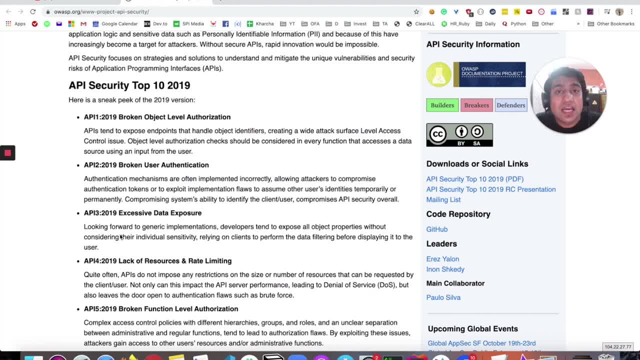 there may be a time when we have to do api, uh, api security checklist. uh, if api security testing, i need to say that. so that's uh where you can keep in mind. these are the top uh 10 secure uh api testing test cases that you need to check right, so you can check for broken. 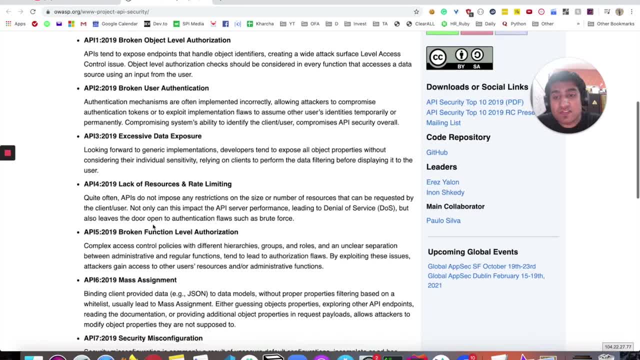 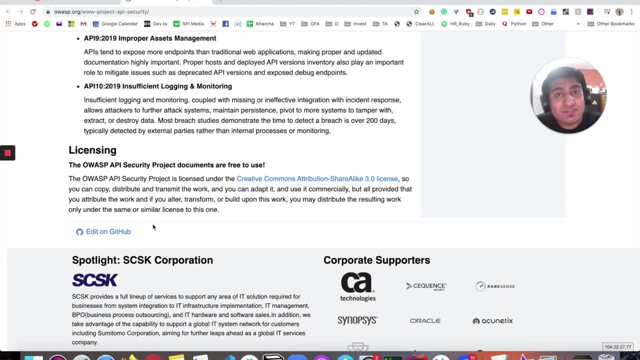 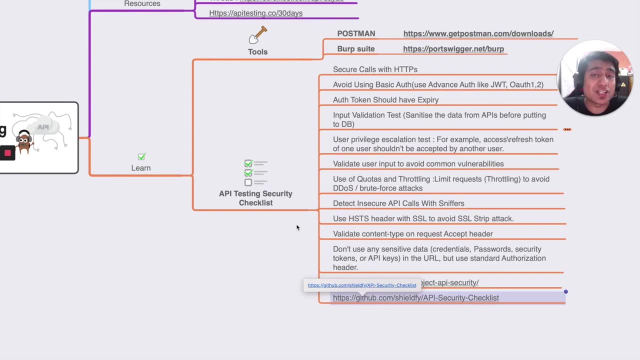 broken object level broker user authentication, excessive data exposure, injections and all right. so i would recommend you to to basically read this full article we have there. they have discussed everything about it, so, uh, i hope, uh, you have learned something about the api testing security checklist, and i have created extensive tutorial in the previous videos also on, so you can check.